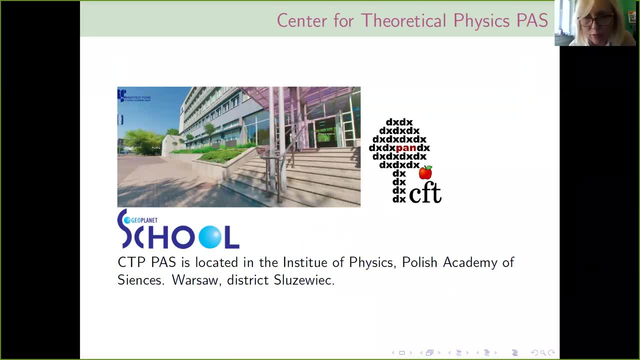 So just briefly about my institute. I hope you can see the next slide now. This is the photo of our building. This is Center for Theoretical Physics. It's located in the Institute of Physics in Warsaw. This is a big campus but we are theoretical division So we share on the 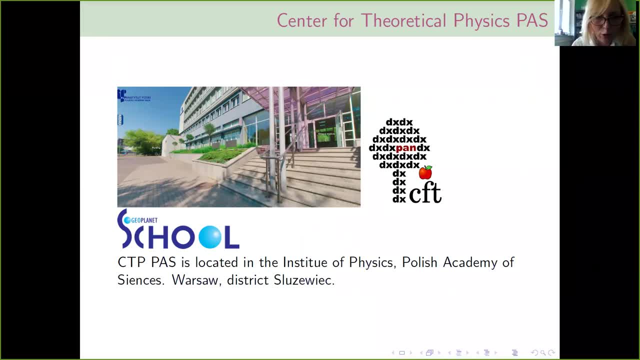 quite a small number of rooms on the third floor on this building And we are hoping to get a new location soon, But at the moment we are here. We are also a member of the doctoral school because as a research institute, we do not lead undergraduate studies. 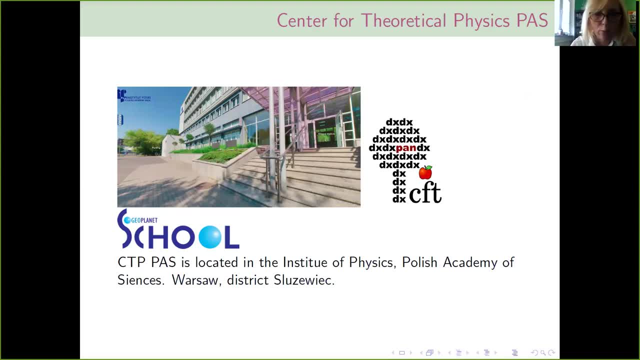 We have only graduate students, And they are members of this Geoplanet School, which is interdisciplinary between Institutes of Physics, Astronomy and Geophysics and Oceanology as well. So I'm in charge of the part of physics here And I have a small group of my own students here. 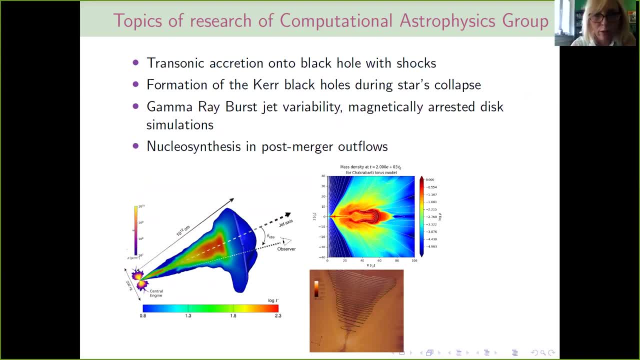 And the topics of our research are related to the computational astrophysics and theory of accretion. So the first topic is the theory of accretion onto black holes. In general, we study different sources where accretion is important, starting from the persistent sources, AGN and X-ray binaries. 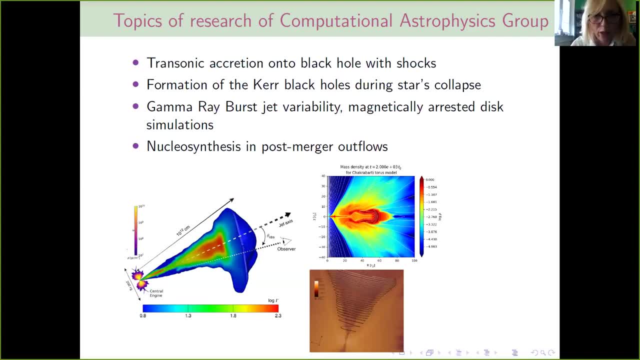 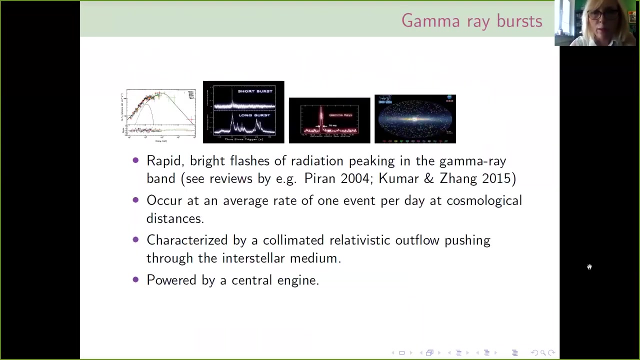 down to the transient and very short explosive events like the gamma-ray bursts. We study formations of the Kerr black holes during star collapse with numerical simulations. We also study gamma-ray bursts in the context of the jets And finally, the nucleosynthesis in the post-merger outflows from the accretion disks. So the topic of today is the gamma-ray bursts. 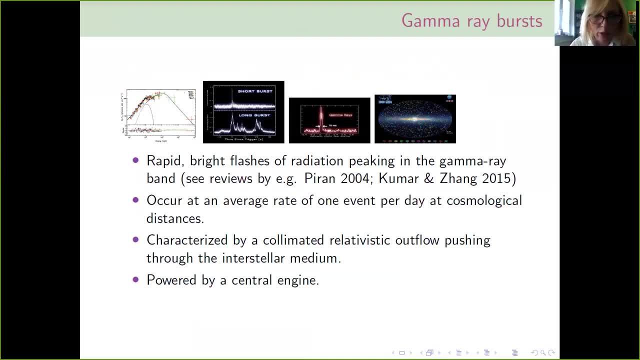 as we heard from Zvi Piran already this morning, The gamma-ray bursts are very powerful energetic events that I observed because of the collimated relativistic outflows are pushing through the stellar medium from very large distances, from extragalactic cosmological distances. 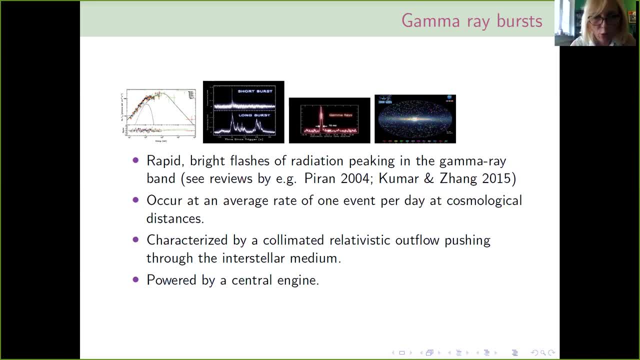 This gives us information about the power of energy released in this explosion. This must be very high, So they are presumably powered by a central engine. This can be a black hole of a kind of a stellar mass surrounded by some remnant matter, And the power of accretion is typically considered sufficient to power the central engines. 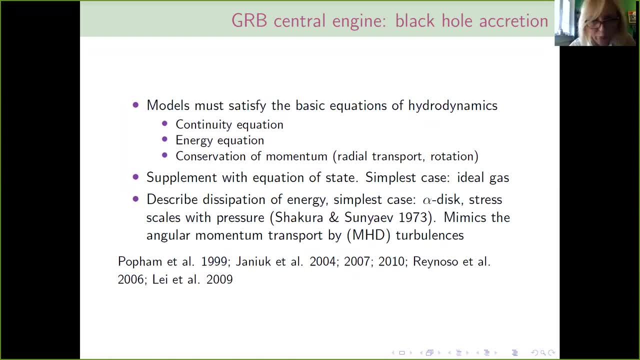 I divided my talk today into two parts. The first part will be a little bit historical and pedagogical information about the problem of the microphysics in these accretion disks, because for you maybe it is very well known, but for people who 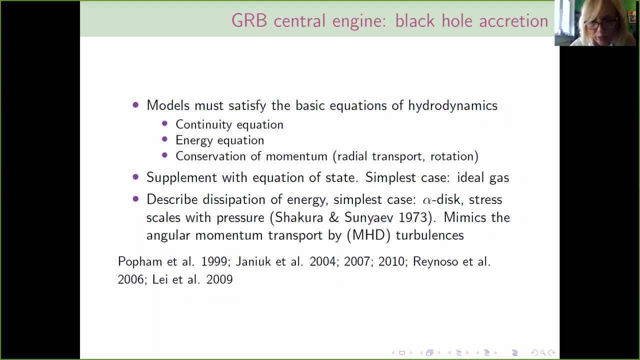 are considering accretion in the active galaxies or in the x-ray binaries. they do not know much about this problem and the microphysics is completely ignored. So here we have a specific model from the 1990s that was based on the standard equations of physics, basic equations. 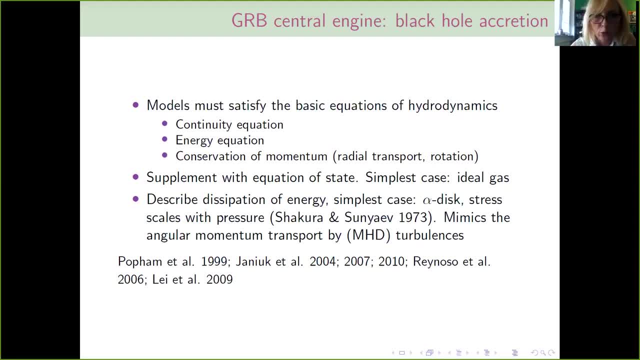 and other equations, And these equations are those of hydrodynamics. They are continuity, energy equation and conservation of momentum. These are sufficient to build a successful model, either steady state or time dependent model, of the accretion disk with the famous viscosity. 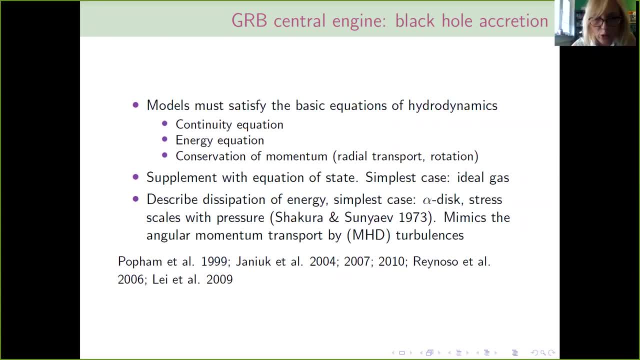 prescription given by alpha parameter, where the stress scales with the pressure, and proposed in 70s by Shakura and Sunayev, But later on it occurred to be insufficient for the description of the GRB engine because, first of all, of the microphysics and the equation of state, where, 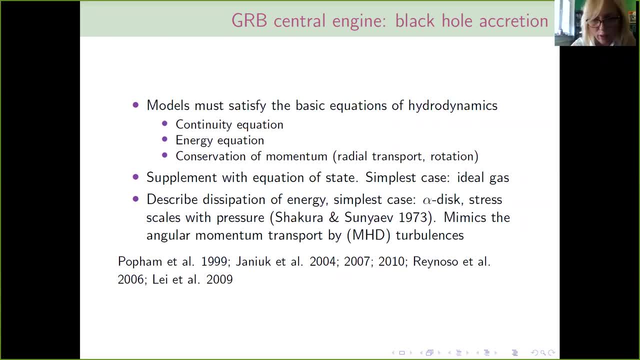 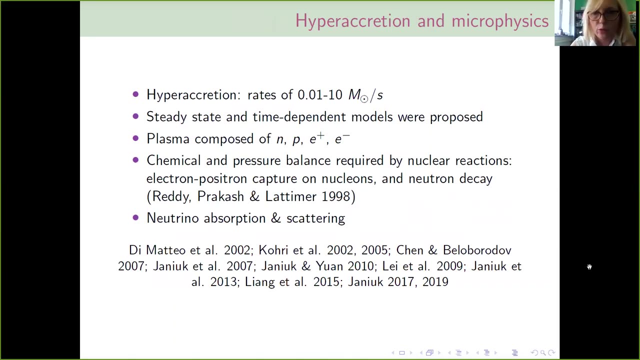 not only ionized hydrogen is important. And finally, going to the MHD turbulences and transport, people started building more advanced models. So in this first part I will describe the hyperaccretion and microphysics in such a simple one-dimensional model. 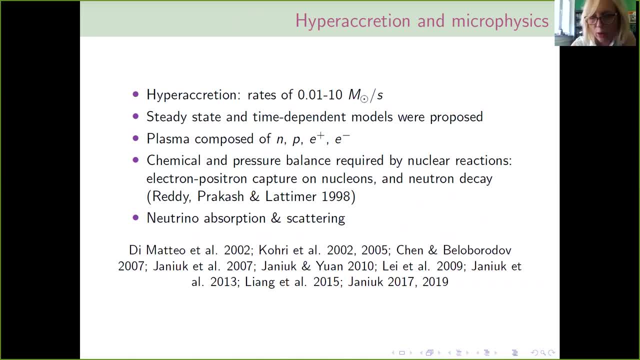 The hyperaccretion is a two-dimensional context of the accretion disk which I studied from the years 2004.. And not only I, but a large group of people- different groups- were involved in such studies, And in the last part of this talk I will show you my recent efforts and the simulations. 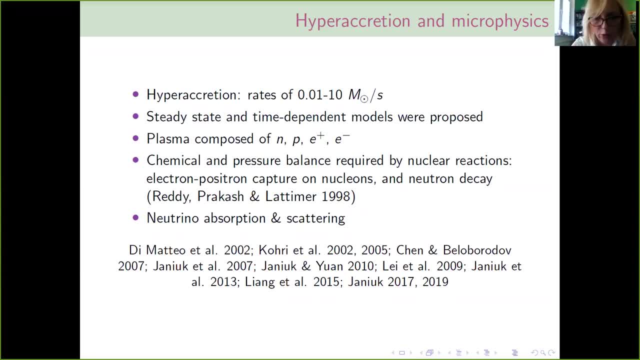 with much more advanced code of general relativistic MHD, which is called HARM. And so what is hyperaccretion? Hyperaccretion is a term that describes the accretion process, but highlighting the rate of this accretion to be very, very large. 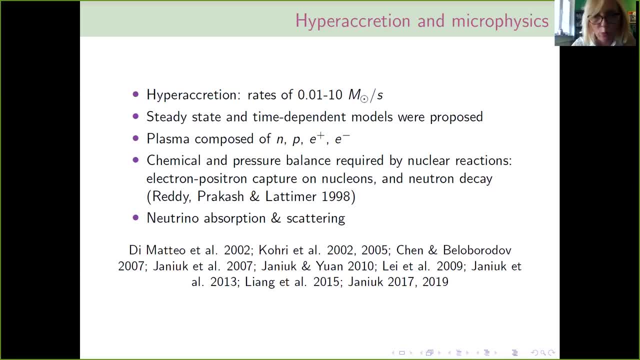 This is of the order of solar mass per second. Specific value is probably more tricky to constrain, but anyway, this is solar mass per second. in comparison to solar mass per year, It is really very high. The plasma here is composed of the ions and heavy. 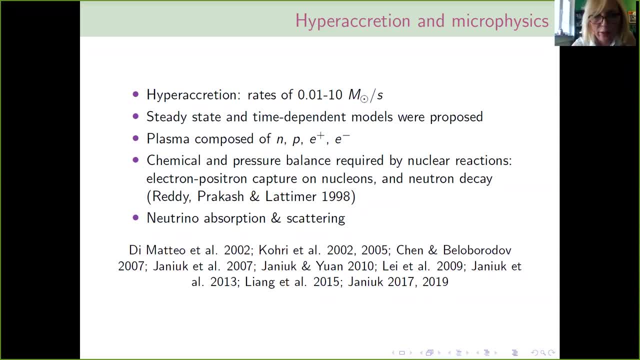 accretion rate. very high accretion rate implies very high densities and high temperatures. That's why these species are free Neutrons. protons, electrons and positrons pairs are also present, And nuclear reactions are occurring here through this plasma, and these reactions produce also neutrinos which can be absorbed. 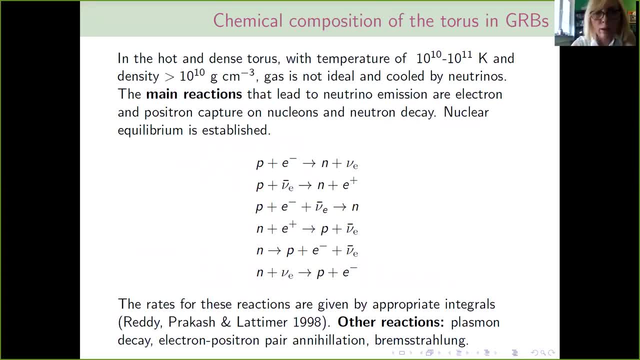 and scattered in the medium. As I said, the temperatures are very high. so these are on the order. 10 to 10 to 11 Kelvin Densities are below the newton star density but still they are very large, higher than typically: 10 to 10 grams per centimeter cube, at least at the start. of the accretion process. So, and it's only up to, I mean just one form. it doesn't always failed. it's a more comfortable form. It's only up to. I'm not going to use this if you find no function of it. it doesn't every day and I'm just telling you because the piect ist the rise of neutrinos. but other criteria is key here. when neutrinos are high, which is not, 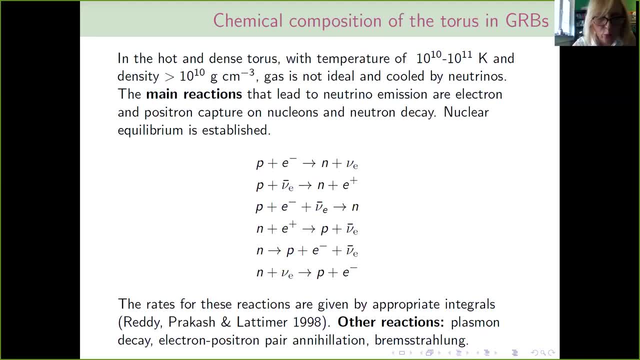 they will gradually drop as the accretion proceeds and the engine is getting empty. The main reactions that produce here neutrinos under such densities and temperatures are the electron and positron capture on nucleons. neutron decay, and between these reactions nuclear equilibrium is established. 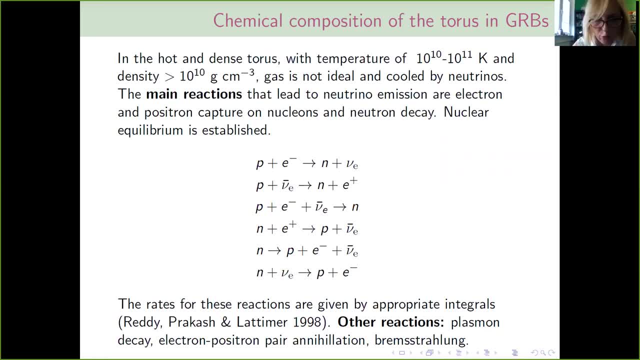 The rates I will show in the next slide. the formula for them were derived in the works by Latimer and collaborators. There are other reactions important here as well and considered also by people to construct the equation of state. These are: plasma decay, electron positron pair annihilation. 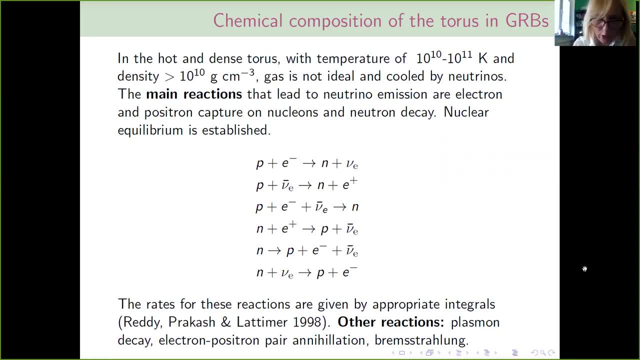 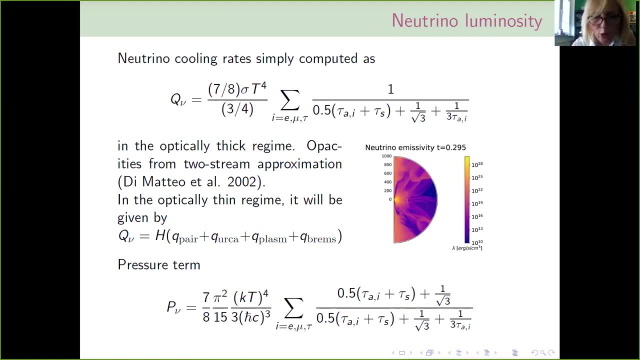 and also branched traluke. so nucleon-nucleon branched traluke can produce neutrinos. There is a neutrino transport problem and neutrino cooling rates or leakage schemes are recently involved. What I have here is very simple: the most simple prescription for the neutrino cooling. 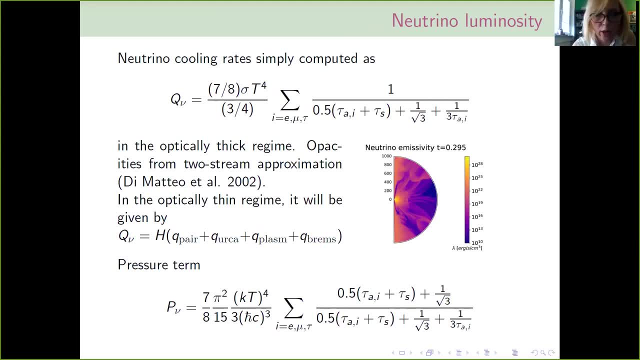 So here the emissivity is computed either in the optically thick or optically thin regime. The plasma actually can be optically opaque to neutrinos. It was shown on Wednesday in the talk by Ariadna. so really in the most densest parts the neutrinos can be absorbed and scattered. 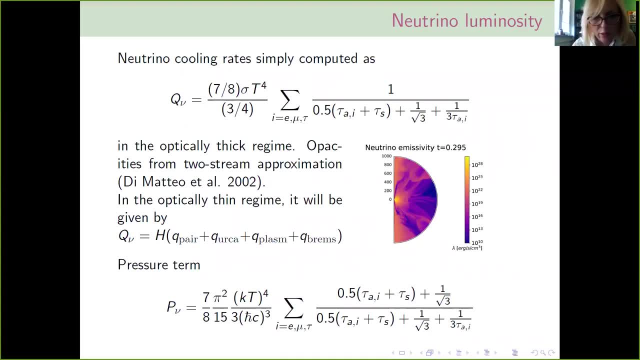 and even contribute to the pressure term given here in the bottom of this slide. I was using in my thoughts the opacities computed from the two-stream approximation given by Tiziana Di Matteo 2002.. This is working approximation and the most simple that we can use. 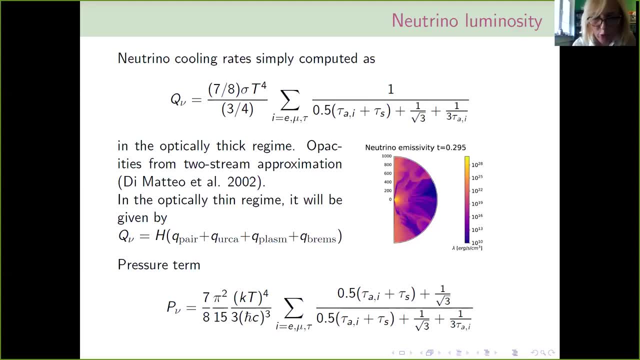 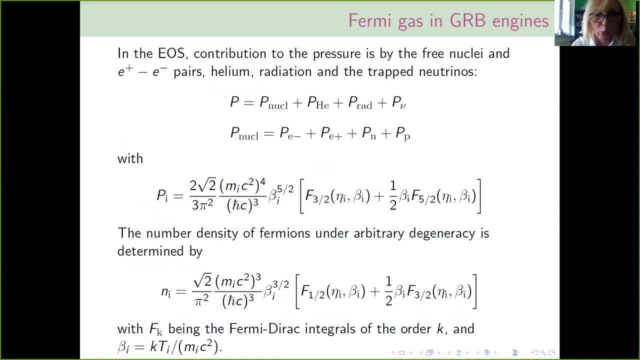 Of course more advanced methods are used now, for instance the leakage schemes, Then the equation of state. The contribution to the pressure is by the three nuclei and electron-positron pairs. Also, helium can be synthesized here in the outskirts of this disk. 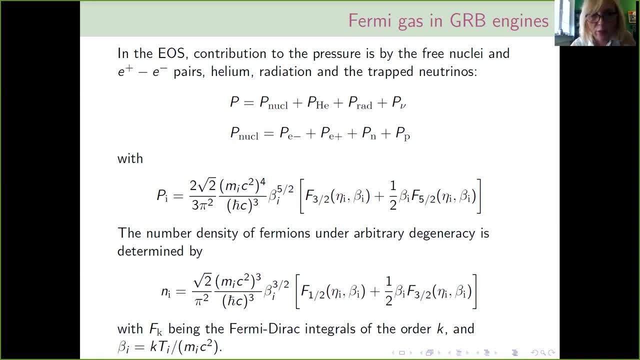 I will show the figure in the next slides where it is synthesized, Radiation and neutrino pressure can be of some importance, but typically they are much lower orders of magnitude. So this is a picture. Fermi gas in principle, with the nucleon pressure contributed by the electrons. 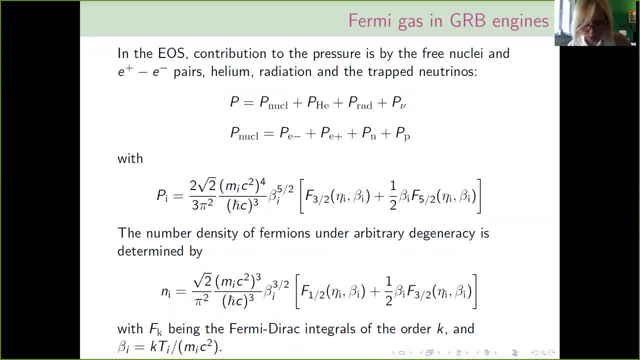 positrons, nucleons and protons, because this fermionic gas has to obey the Pauli exclusion principle, and hence we are computing not the ideal gas pressure in general, but we compute the pressure given by the Fermi Dirac integrals here of the order 3 over half and 5 over half. 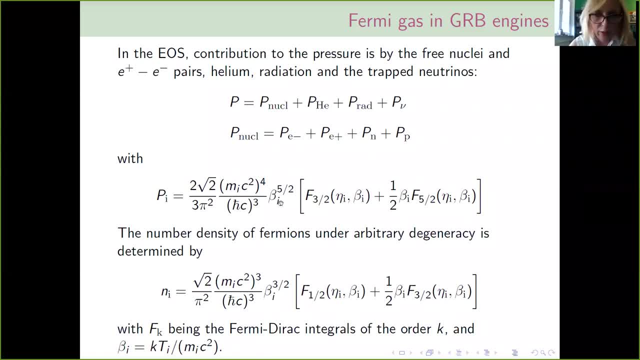 Here the beta is the kT over mc2.. This is the Planck constant here and physical speed of light. So these are computed numerically. And also number densities of these fermions under arbitrary degeneracy can be computed and these are determined here by this formula in the baton. 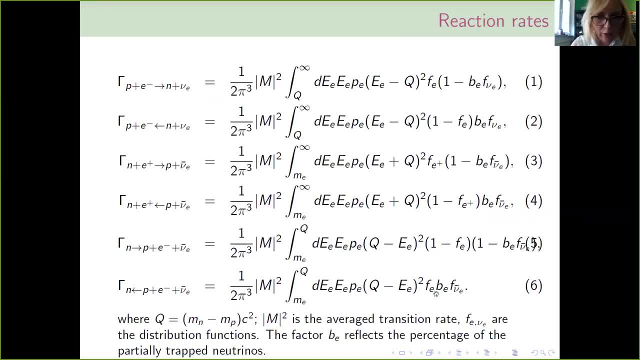 Here you have the rates. They look horrible, but in fact these are three reactions. here, If you look more carefully, there is arrow right or arrow left. So these are reactions back and forth, producing neutrinos or absorbing neutrinos, And here these are integrals over the distribution functions of the species. 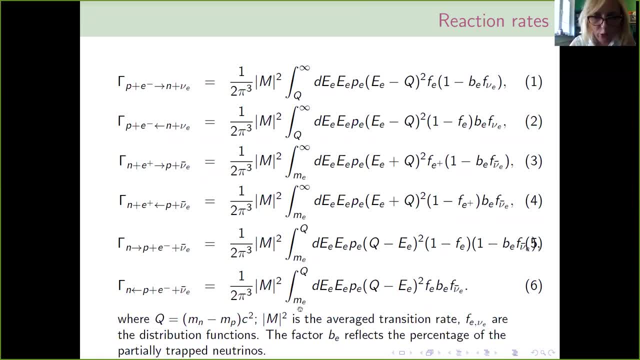 The m. large m is the average transition rate that comes from the weak interaction Catholic constant and is given by the most recent data from the nuclear physics people And the factor Be. here this is denoted. it reflects the percentage of the partially trapped neutrinos. 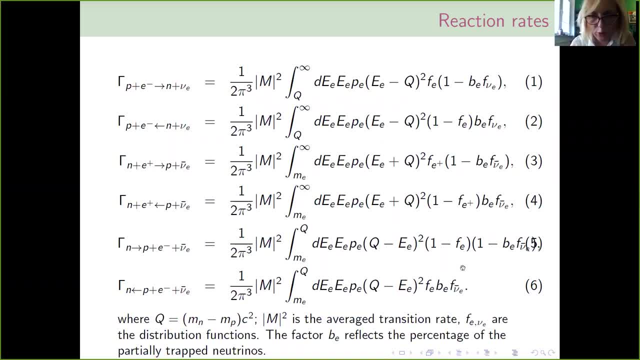 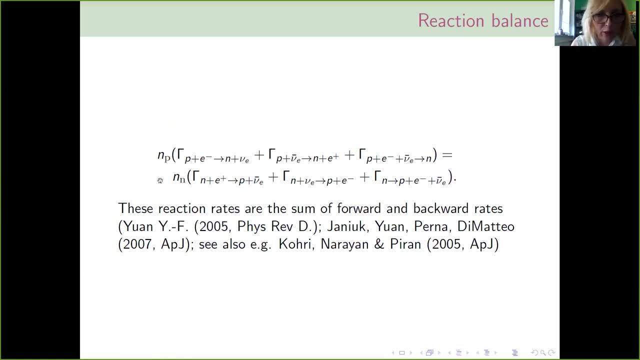 So this is the blocking factor for neutrinos used Here. it can be between 0 and 1.. The reactions have to balance each other. Yes, so this is the number density of protons versus number density of neutrinos, And reactions which consume protons have to be balanced by these which produce them. 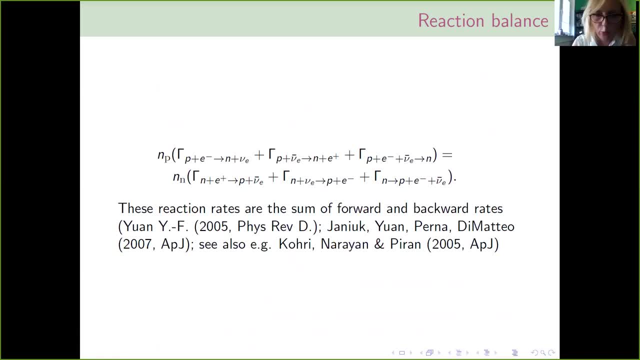 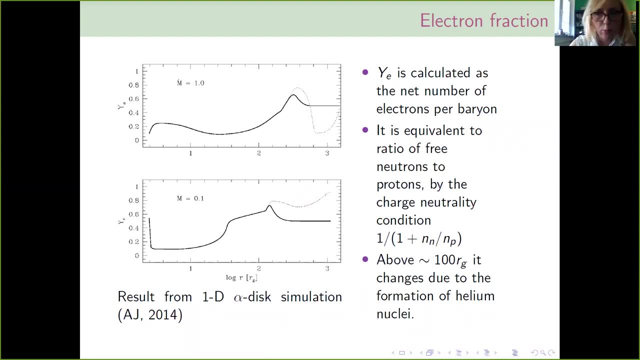 And from this kind of balance we just compute the electron fraction. The electron fraction is calculated as the net number of electrons per baryon. It is shown here on the slide. This is the plot. This is the result from this 1D alpha disk simulation that I made 2014,. 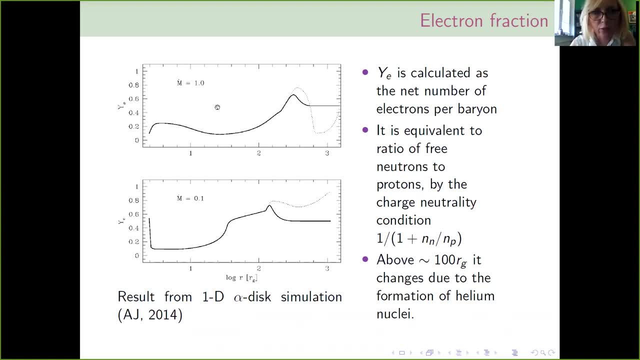 so quite a long time ago. But the parameter here that sets the physics conditions is the accretion rate. I have plotted two examples here. the accretion rate: 0, 1 solar mass per second and 1 solar mass per second. 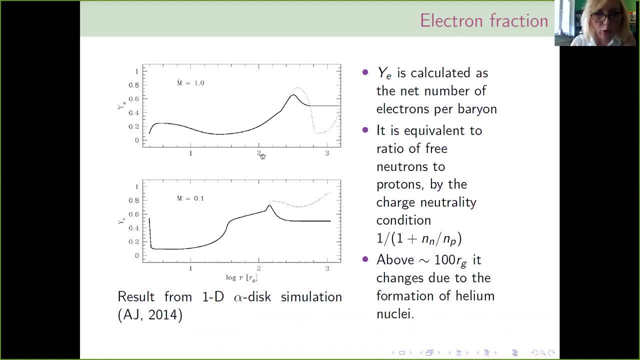 And you see that in the large part of this disk this is log scale of the radius up to 1,000 gravitational radius. this electron fraction is pretty low under such conditions. So this is even below 0.2.. And above 100 RG. you see, here something happens. 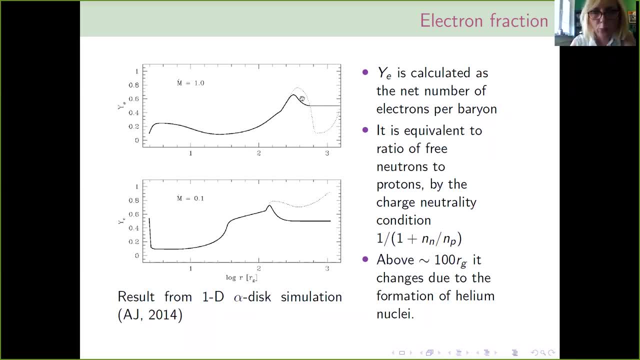 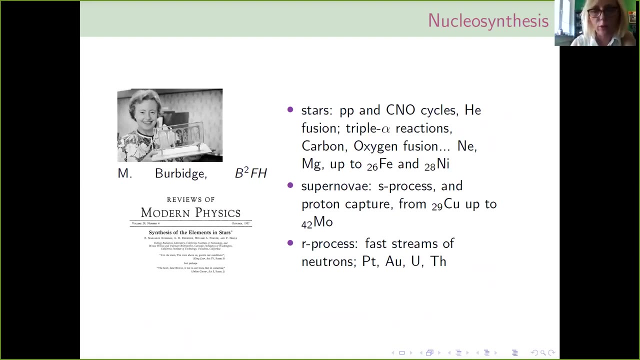 So this is the place where helium is being synthesized. So these electrons are also then in the helium nuclei. Okay, what about nucleosynthesis? I use these models for different purposes Also. I think it's kind of useful actually to go back to these one-dimensional models. 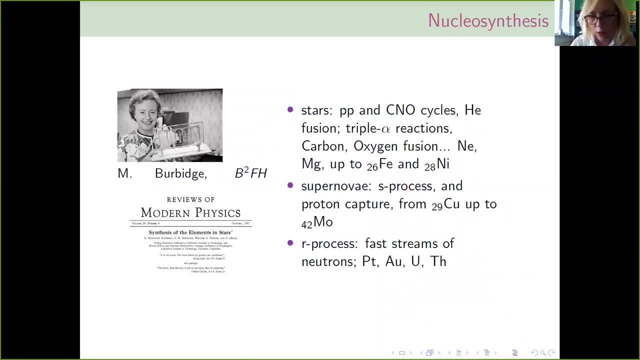 for pedagogical reasons, to teach students how the physics looks in quite simple simulation that is possible to be done on the laptop. But also it's interesting from the point of view of problem of nucleosynthesis in this accretion disk, Because what we know from the history of physics 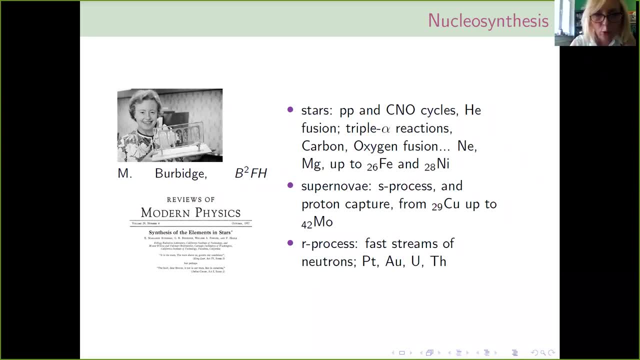 we know that in the past we have seen some very interesting phenomena, For example in the case of this seminar work by Barwich, Barwich, Fowler and Hall from 1975, it's been over 60 years now the anniversary of this work. 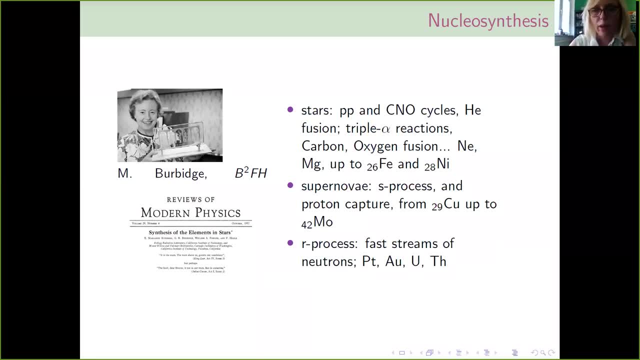 They showed greatly that stars produce helium and carbon oxygen. in the fusion The elements up to iron and nickel are produced. So we can get heavier elements And from starting from these elements synthesized inside the star, we can get heavier elements in the explosion of the supernova. 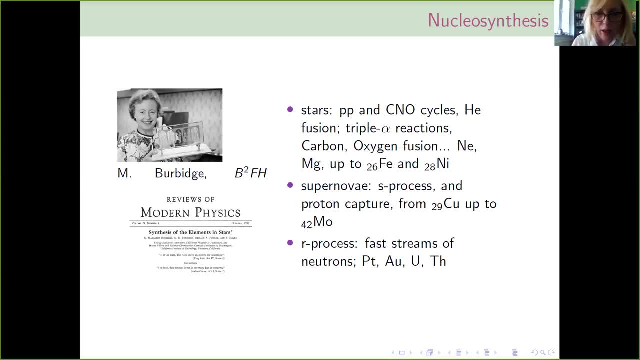 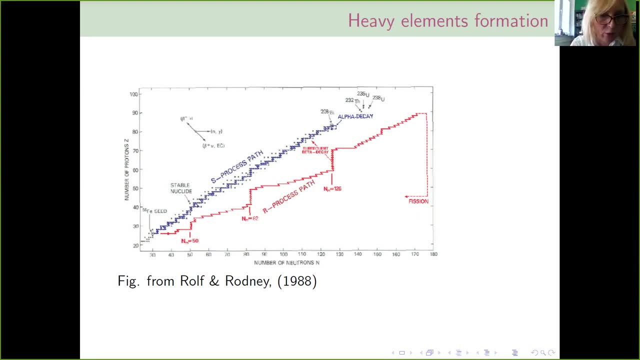 Then the R process is needed to explain the fast, the heaviest elements produced in the fast streams of neutrons. So you see here these chains on the diagram of this. number of neutrons versus number of protons in a nucleus Is represented here on such a stability line. 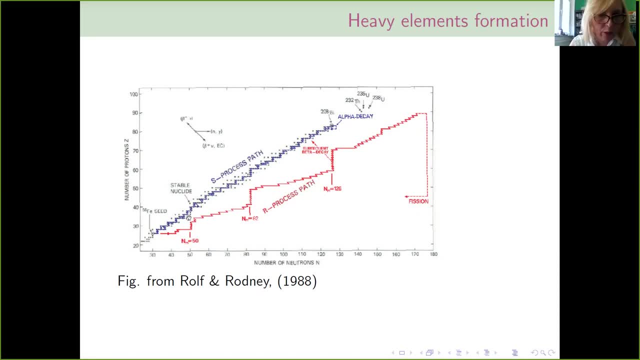 Yes, these are the elements that the isotopes synthesized or produced by two different parts: S process and R process. So you see from this textbook figure that heavier elements are only possible here on the top right of this graph, by the R process path. 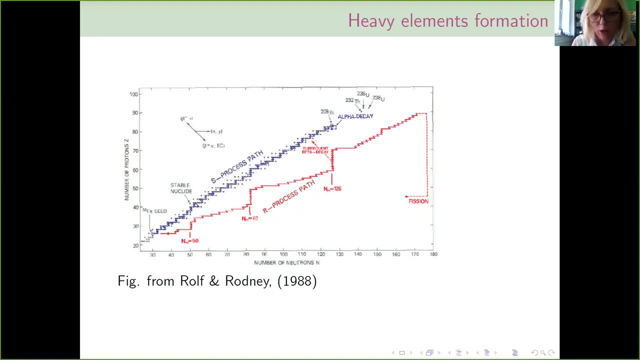 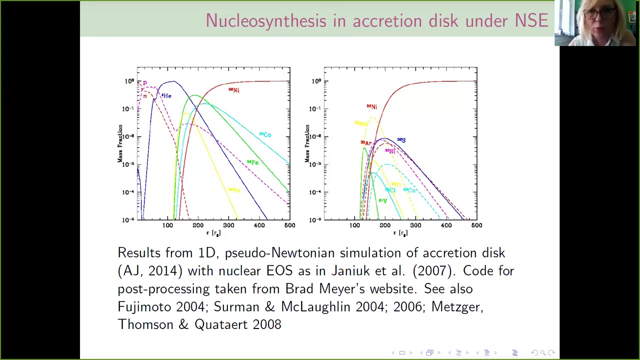 Is it possible, then, to apply such idea to accretion disk? This was curious for me because I'm accretion disk person. I was not working on stars before, So I just wanted to see if the nuclear synthesis can happen in the accretion disk. 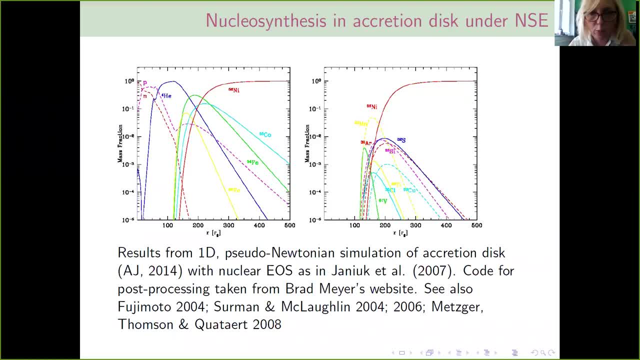 And first I started from this nuclear statistical equilibrium. There is a method, well established and available, to use this code for post-processing. I've taken from the Bradley Meyer webnuclearorg website and he provides quite a nice toolkit for it, And this is the post-processing result of my one-dimensional simulation. 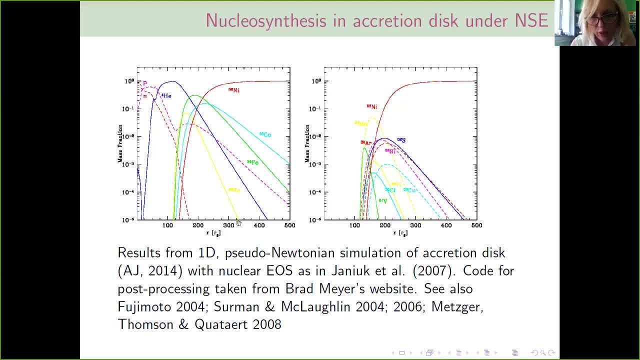 of the steady state accretion disk, alpha disk simulation. So here you see how these species are distributed inside the disk. So of course, as I said, you have in the innermost part only the free protons and neutrons. 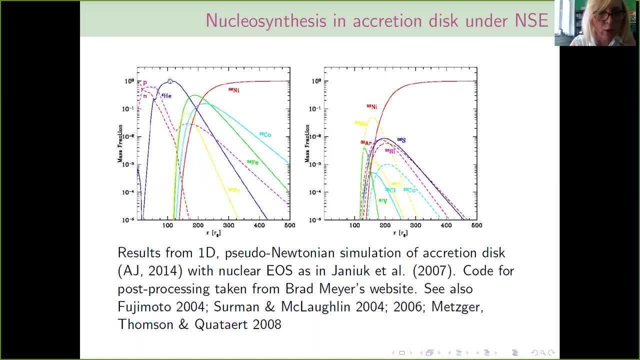 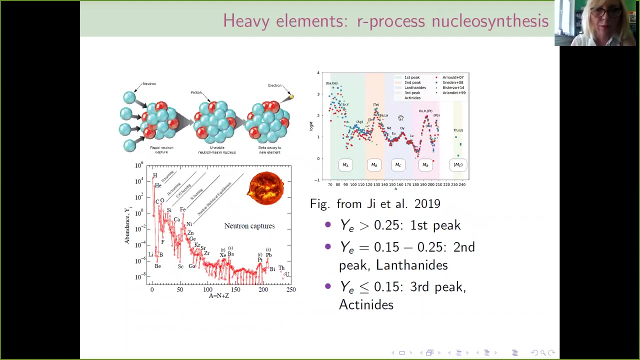 As before, then this helium is forming, Yes, around 100 gravitational radii. It's a peak, So the mass fraction is dominated by the helium. But then you are having more and more heavier isotopes synthesized, But of course only until nickel, because it is an acid thing. 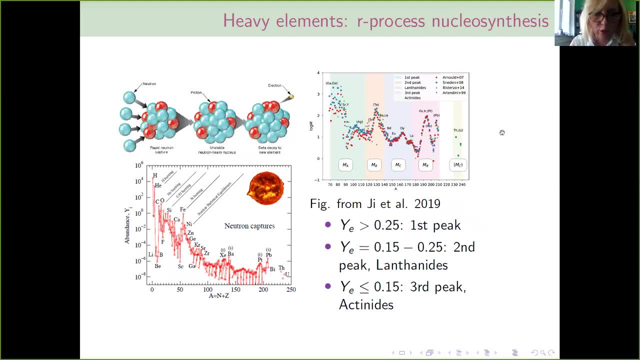 Heavier elements than nickel, of course, are produced in the universe, And we see this here. Yes, we see this. Nickel is the abundant, the last abundant element that can be produced under NSA conditions, But then these neutron captures produce all the family of much heavier isotopes. 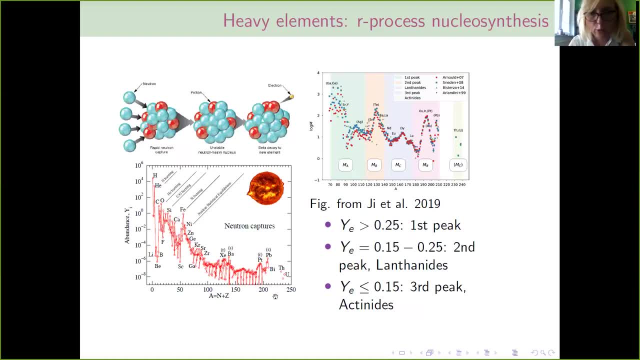 with much larger mass numbers. Here you see the graph how the R-process and rapid neutron capture looks like from the point of view of a single nucleus. So it has to be put into a batch of neutrons with large number density And these neutrons are attacking our, our nucleons. 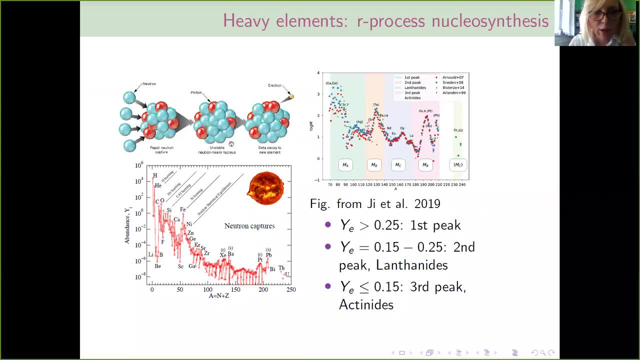 There is unstable neutron heavy nucleus, first at the intermediate stage And then there is a beta decay And the nucleus goes to the virus. There is a value of stability back on the line of this R-process And what is important Is this YE. 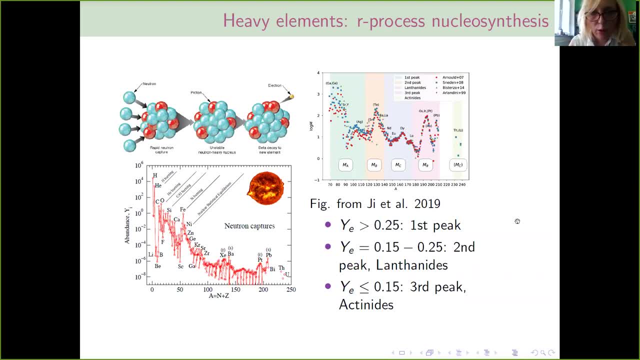 Yes, this is the electron fraction condition. How can we form heavier and heavier elements? under which conditions? So this figure also shows you what is being produced. And these characteristic peaks may be seen better here than in the solar orbit. So you see here much more pronounced peaks of the first. 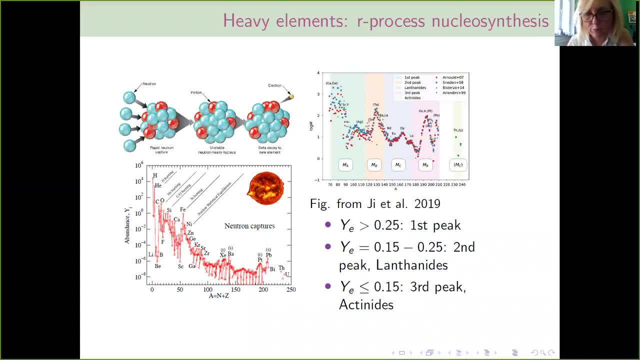 second and third R-process operation And the first peak can be produced if the electron fraction is not so small, has to be larger than about 0.25.. Then the second peak and the lanthanide family of isotopes can be produced only under a much smaller electron fraction, value 0.15, 0.25.. 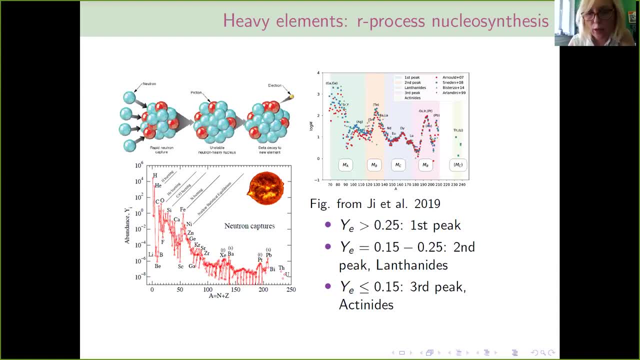 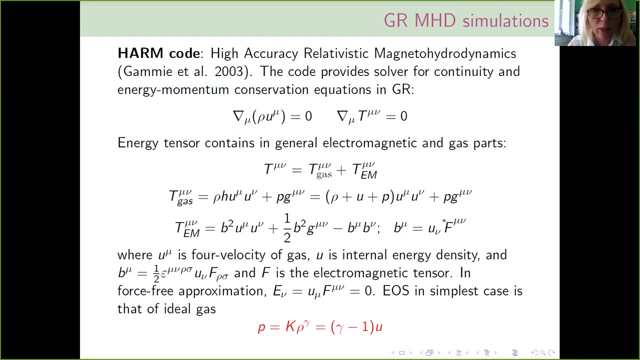 And the third peak requires the electron fraction to be even smaller, And here only the actinides can be traced. OK, so to do this I implemented the HARM code, So you are all very familiar with the HARM code. Here I had a problem. 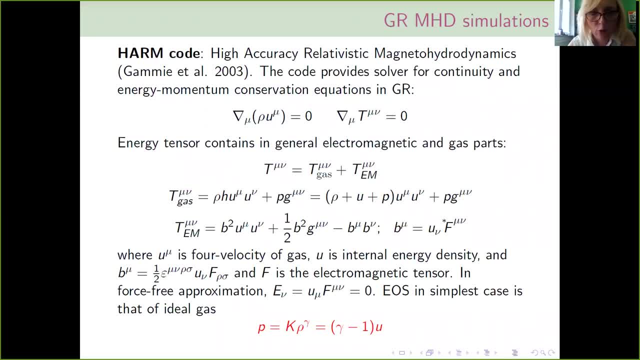 Here. I had a very beautiful lecture on Wednesday by Scott Noble, So he's one of the authors of this scheme, So I don't need to explain to you. The code provides the solver for these continuity and energy momentum conservation equations. but now in general relativity. 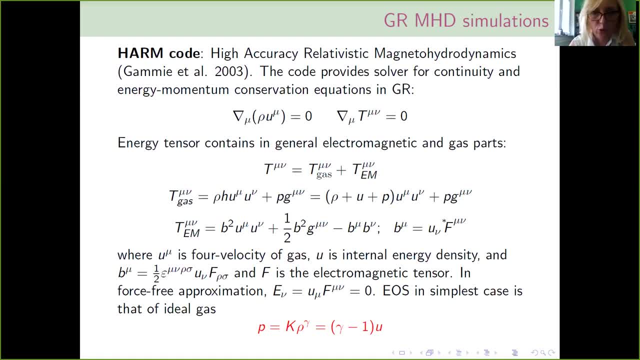 So it's all under the 3 plus 1 decomposition of the spacetime and the matter together with magnetic fields under the Kikset-Kerr background metric, And there is the energy tensor that contains these two terms, the gas and the electromagnetic part. 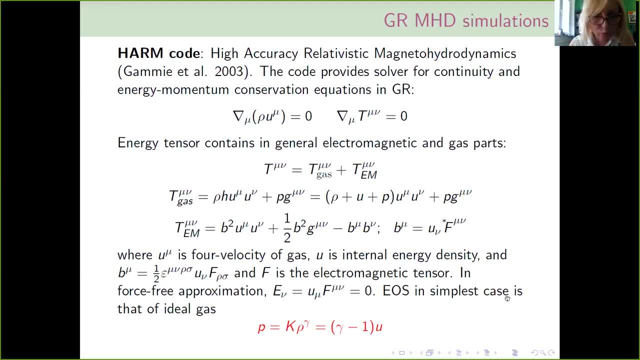 The flow is magnetized And the equation of state in this basic version of the code that is available to download from the first. I started with this version from Charles Gamy 2003.. This provides the equation of state of an ideal gas. 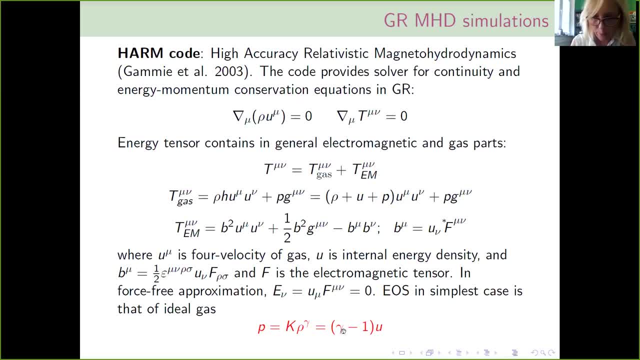 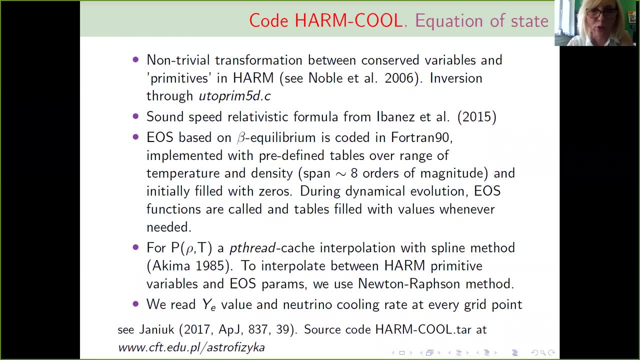 Here the gamma is the adiabatic index. So what is needed to implement the microphysics into the HARM code? I needed to really go inside the code and look at the inversion schemes between the primitives and conserved variables in HARM, because HARM is a conservative scheme. 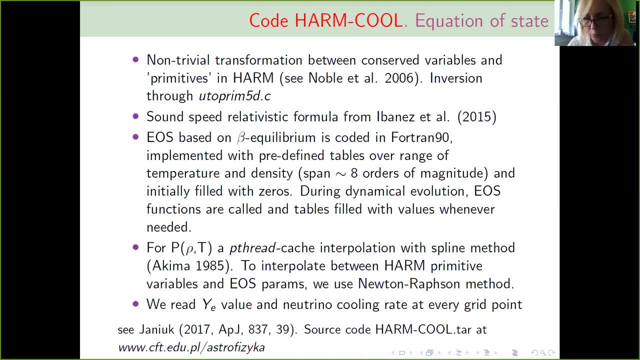 and advances the quantities, such as total energy or the co-moving density, Why we have in the EOS computation we have a rest mass density and temperature. So we need to transform between those variables at each time step And for that really it is important. 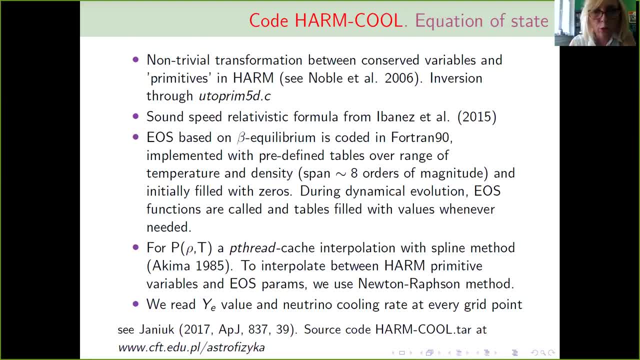 which routine you are taking. We have to take this utoprim 5D because it's much more accurate. So people familiar with the code already know which is the one, because there is 2D and others, but only this 5D worked. 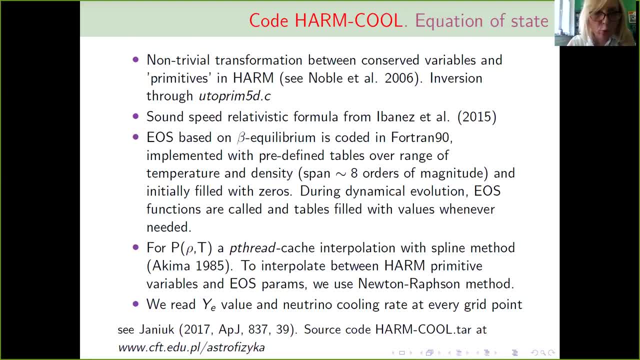 The sound speed is important. So you have to consider relativistic formula I took from Ibanez. I know that Scott took another one, but still the one that was in the default version was not good. So I have the code for the equations. 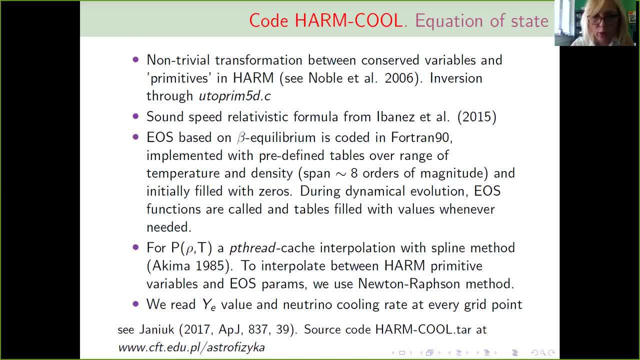 of state based on this beta-equilibrium. They are routines in FORTRAN 90 that are implemented here into the HARM with special, just into the make file And they are implemented in such a way that we predefined the tables over a range of temperatures and density. 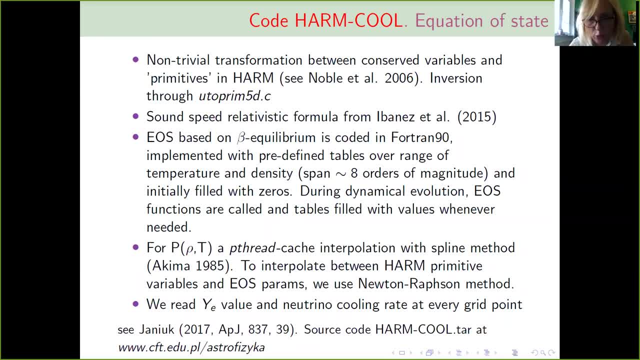 They are spanning at least 8 orders of magnitude for each, just to cover all the floors of the code and let the code evolve from the initial conditions, And initially we fillet these tables with zeros. During the dynamical evolution, the equation of state routines are called. 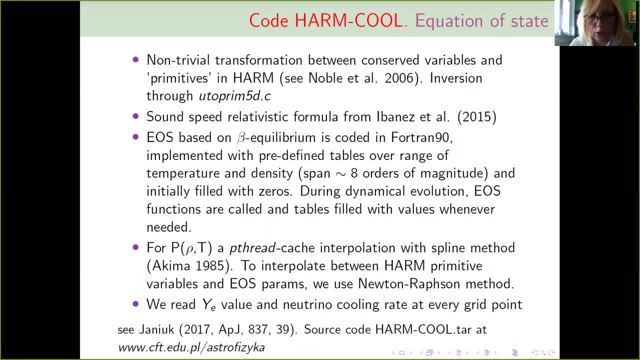 and the functions are called only whenever needed, And then the tables are filled with these values of the pressure and the neutrino cooling rate and so on, as a function of density and temperature, And of course we have to do some interpolation because of the surrounding values. 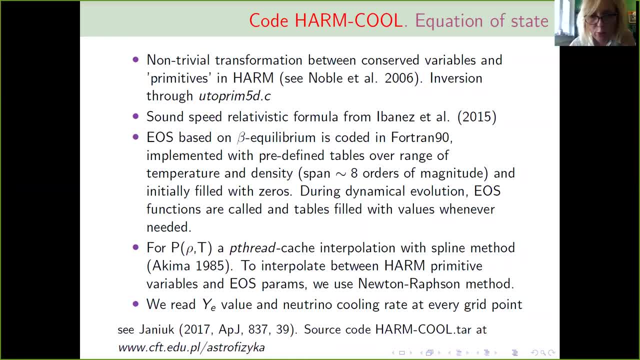 are needed for this interpolation. We store them in a cache and this cache is filled all around one of the cells- There are four- by four other cells and this is distributed in parallel way so that the code is using the generic Linux property, the pthread. 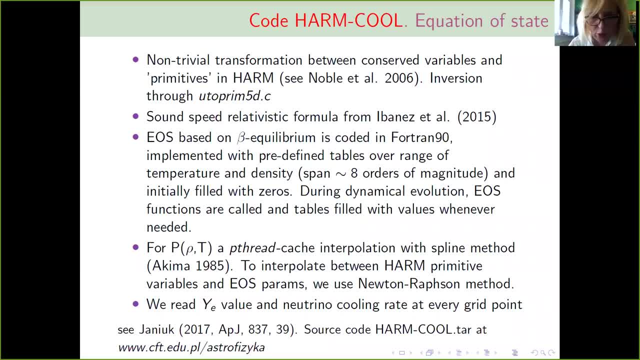 So it's doing this interpolation in parallel way to be a little bit faster. The method used here is given by Akima spline interpolation. Then simply using Newton-Raphson method, we interpolate between the harm primitive variables and the else which parameter values. 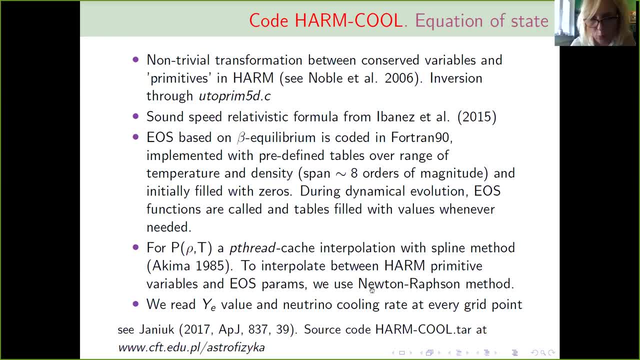 So this is done in not so very difficult way. Two minutes, please. Sorry, do I have to finish In a few minutes? Few minutes, okay. Yeah, I try to be fast. So we read the y-e value and neutrino cooling at every grid point. 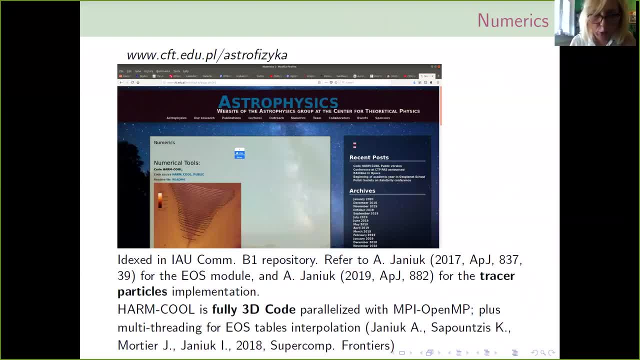 The code is available for free to use. And what I want to say finally- this is last point here- We also implemented the tracer particles in the code. The code is, in principle, fully three-dimensional, It's only that I have to use actually two-dimensional simulation. 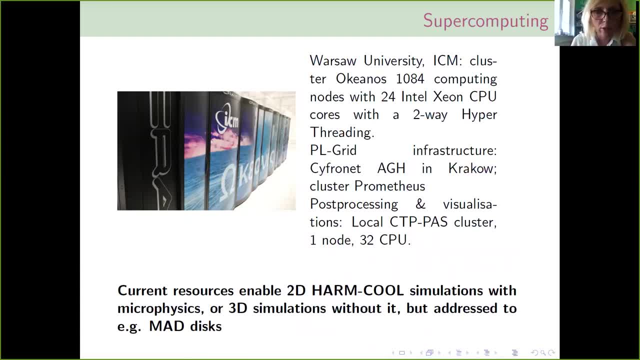 because of limitations of the hardware that I have. This is the hardware. and well, this is a cluster of the Warsaw University Center for Computational Modeling. You can think it is large, but there are a lot of people who want to use it, So yeah, 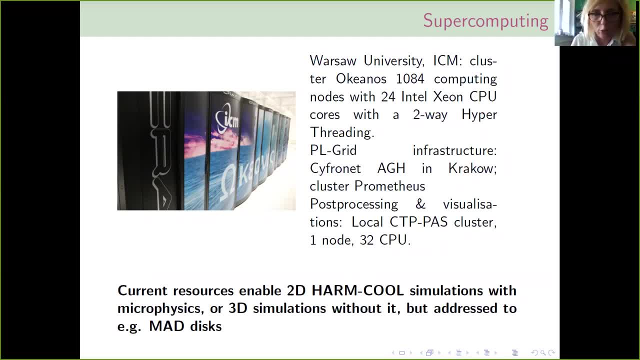 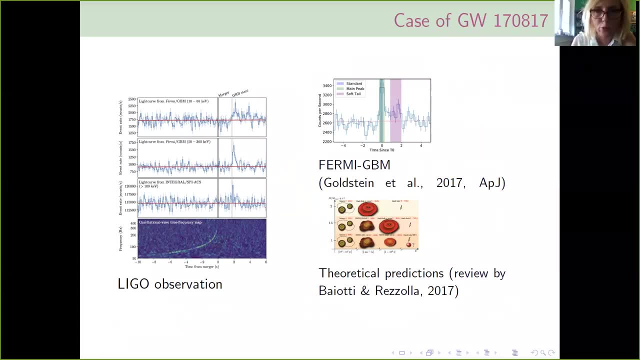 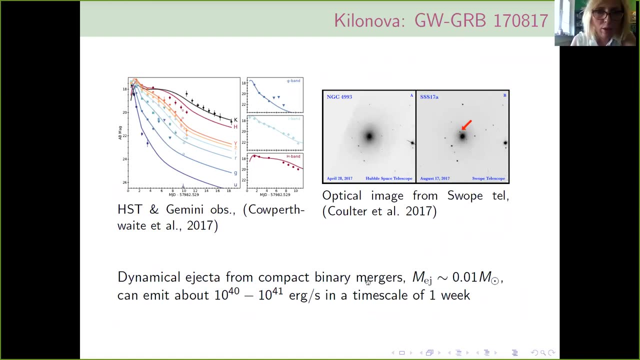 I restricted my models last year only to two-dimensional setups, And the motivation, of course, to publish some work about this was the discovery of the GW1708 kilonova, So I don't want to repeat what was said before about this, just to show the image. 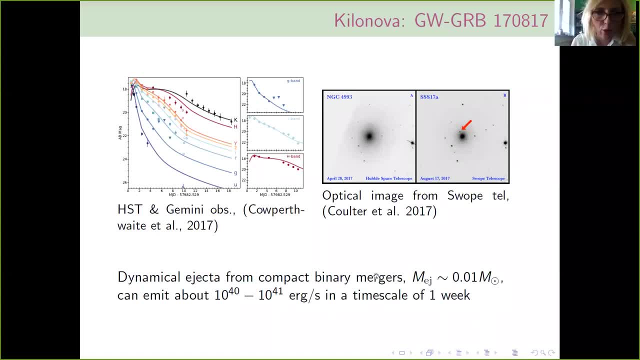 This is optical image on the right here of this kilonova And this is the kilonova light on the left. So you see this. different components, red and blue, And it is supposed that the dynamical ejecta from the mergers are supposed to be responsible. 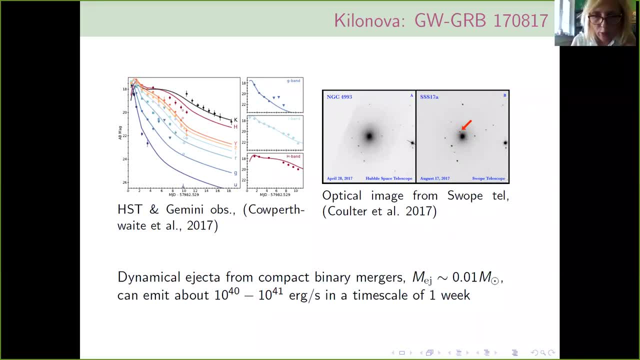 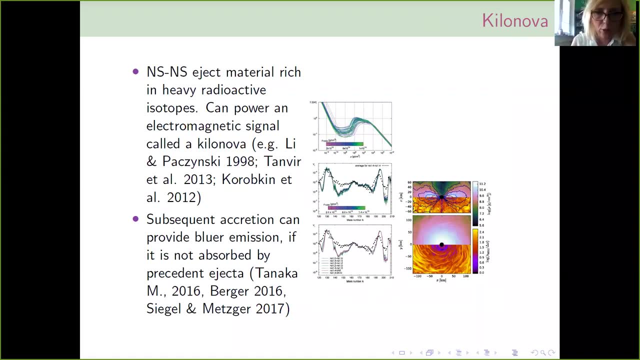 from the timescale of about one week to produce this kilonova. But also it is thought that subsequent accretion can provide bluer emission And if it is not absorbed by this dynamical ejecta from the merger, it can be revealed later on with time. 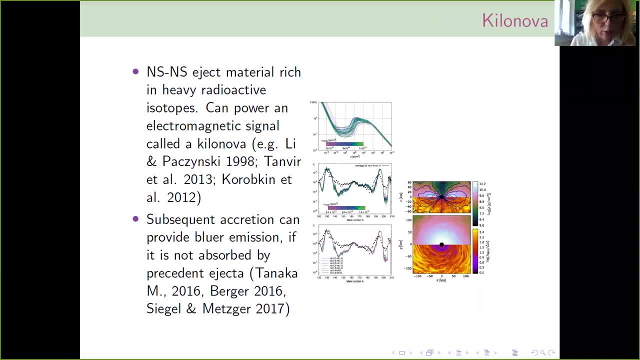 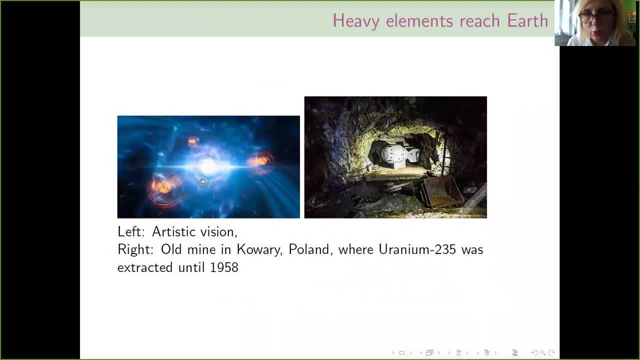 And it was discussed also by Daniel Siegel yesterday at this point. So okay, I will just skip this. This is just artistic vision. Yes, that we have this kilonova explosion. We have this signal about a couple of weeks after the gamma reverse. 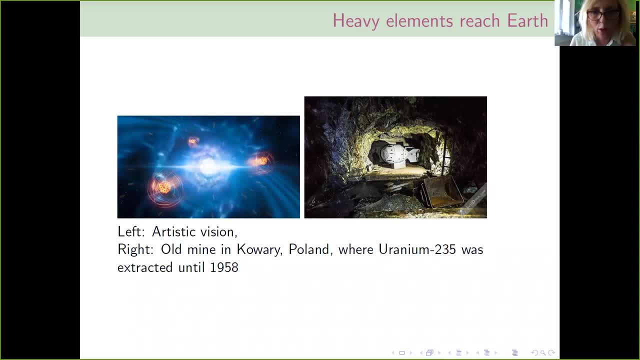 and the gravitational wave observation. But then we have also remnants of this traveling through the interstellar medium and reaching the solar system. Actually, the elements that are reaching us are not only gold and platinum, to produce the jewelries, but also heaviest isotopes. 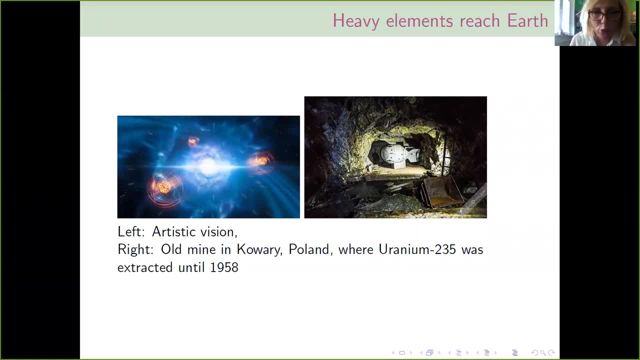 for instance, uranium can also be produced in such an event, And here is the photo that I took visiting the old uranium mine in Poland. Now it's a museum there, So you can see only a model of the uranium bomb. that is now fortunately not in use. 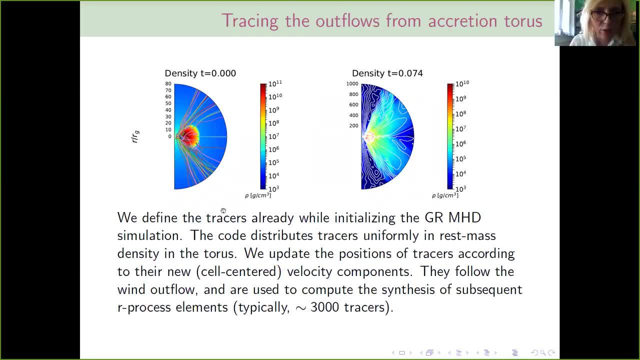 Okay, and about the tracers? This is the image, the figure which visualizes the tracers And they are distributed uniformly in the rest mass density in the torus. We update the positions of these tracers according to their new velocity components. 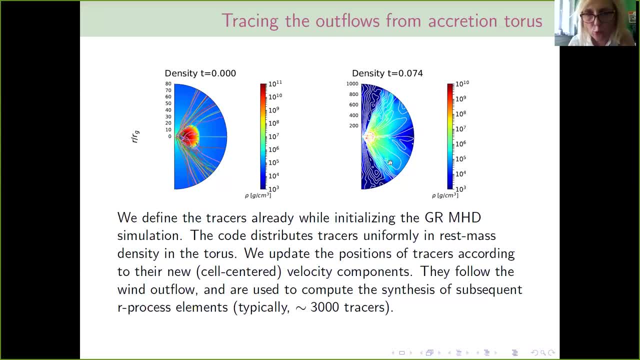 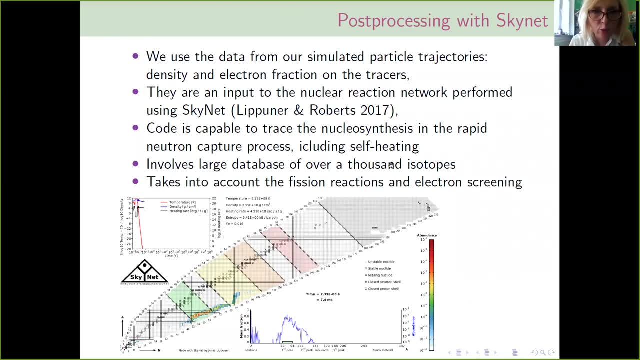 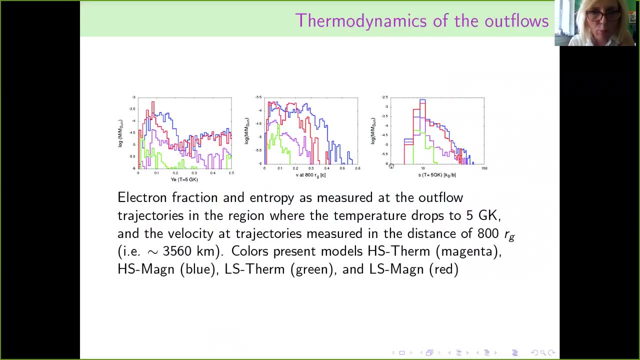 and they follow the wind outflow. The wind is magnetized, as you see here on the right plot. This is the magnetic field distribution in the wind. We use the post-processing with Skynet. I will not talk about Skynet because it was a talk before about this. 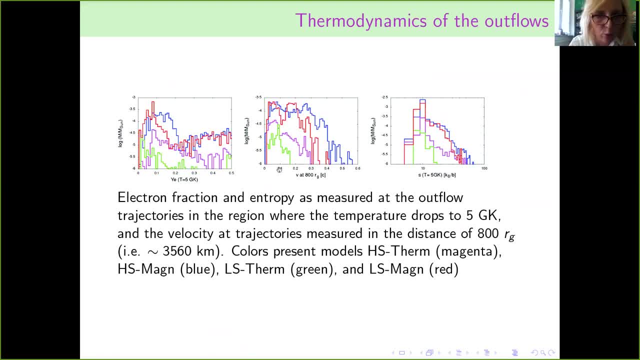 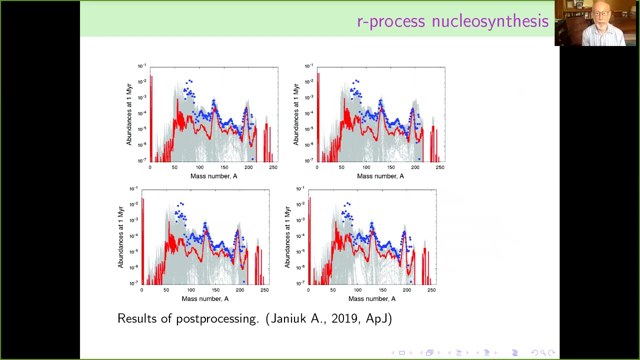 So this is the result. electron fraction distributions in the mass bins. Yes, on the left plot, On the middle plot, there is a velocity distribution of this ejecta that we produce in the wind and trace with the nucleosynthesis code. These are the results showing the abundances. 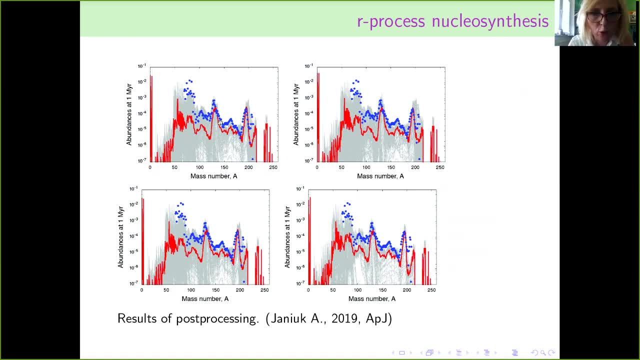 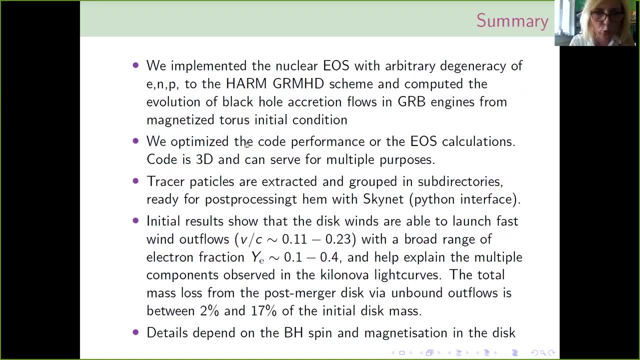 as a function of mass numbers. So you see, the red line is a model, The blue dots is a solar abundance pattern And you see the peaks of the R process are being reproduced. So this is a summary of my talk. I hope I'm not too long. 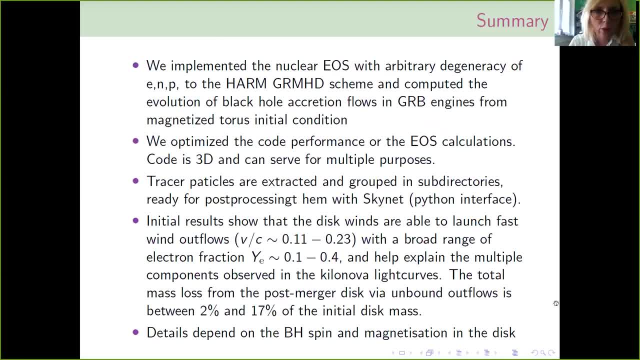 So I just leave you with the summary. Basically, the result for science is that the wind outflows that we have here are having velocities of 0102 of the speed of light, and the broad range of electron fraction is produced. This is why E in the range of 01 up to 04.. 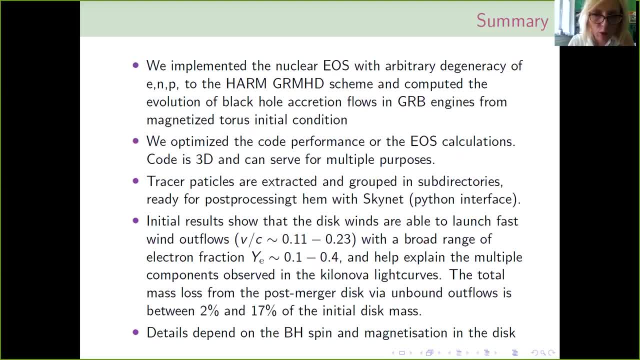 And this, we can envisage, would help to explain the multiple components of the kilonova light. As for the mass of the post-merger disk and these outflows, they are quite small, between 2 and 17% of the initial disk mass. 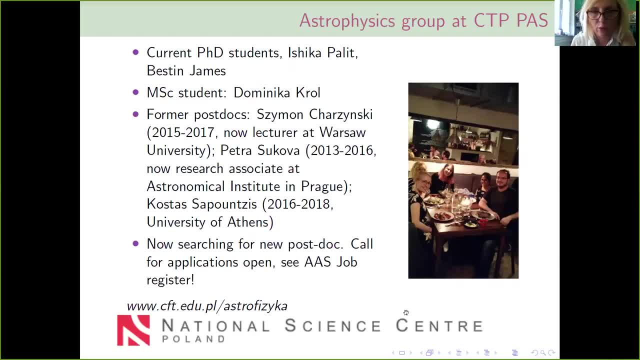 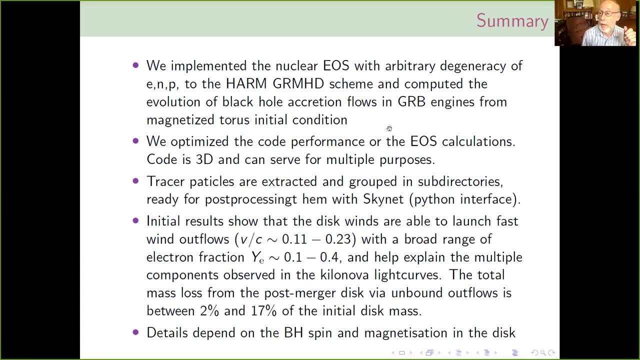 But all of this depends on the parameters and is hard to constrain. So now I want to just say thank you and wait for your questions. Does anyone have questions? Please don't hesitate to ask the question. I'll just ask on the mic. I don't think we have any more questions. 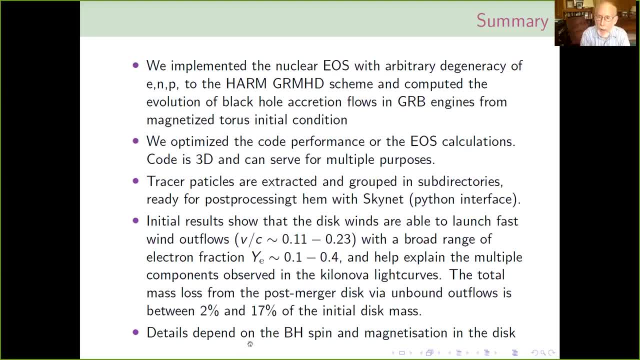 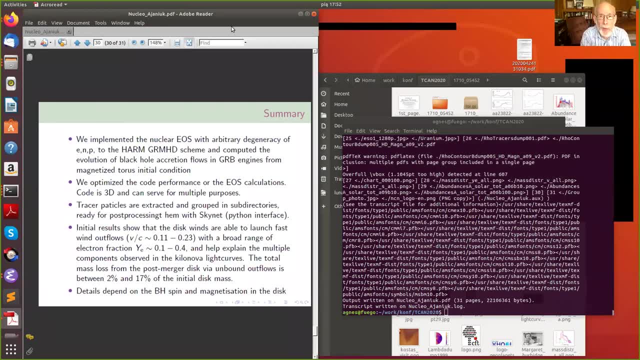 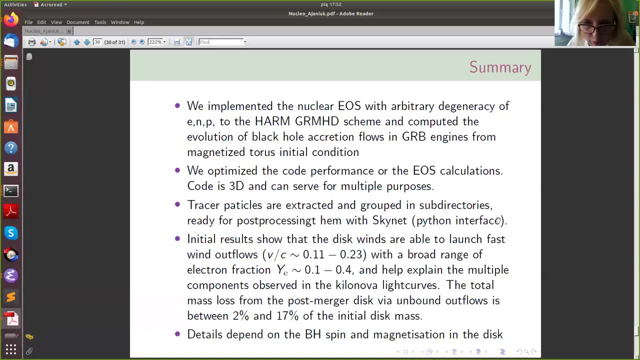 So I will just leave this open to the chat. Thank you, Just to ask: how different are your results from people who have done similar calculations? How different? Well, I think quantitative differences are here present. For instance, the total mass loss from this ejecta is kind of small. as I said, 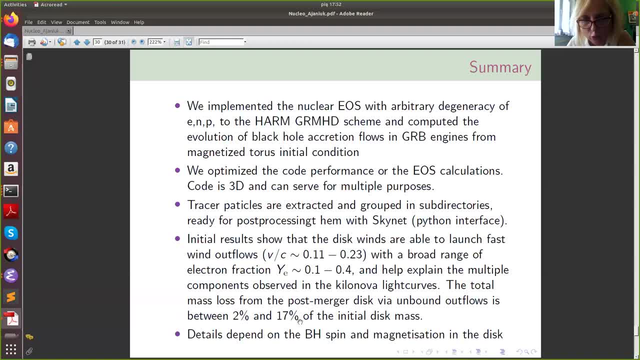 I think people could have higher masses of the outflows. So this is one point. As for the electron fraction, I think this is the broad range that we have. I know that Rodrigo Fernandez was computing such similar models And he has, I think, larger electron fraction values on these figures that he showed. 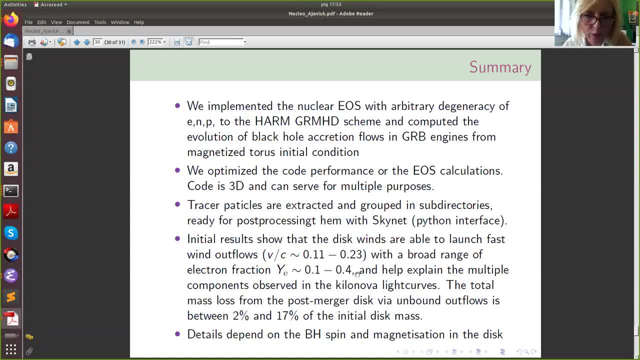 So quantitative difference, of course, are here because of the setup, because of the limitations of this code and all the technical- how to say? imperfections. Of course it could be great to Implement the 3D computation, first of all because it is 2D. 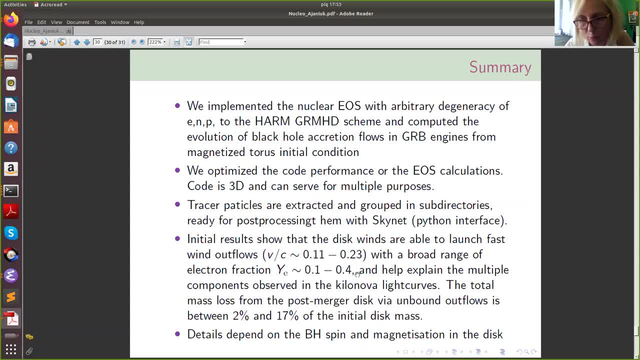 And also for the neutrino transport. this is the biggest challenge. All right, Are there any more questions? Ah, Francois. Yeah, I might have missed this during the talk. So this is a 2D simulation. How long are you simulating it? 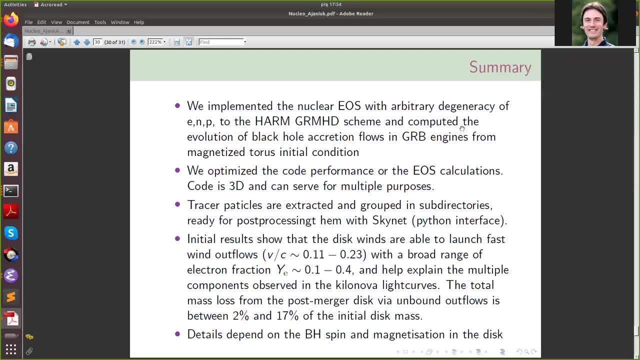 Is it the same kind of length as Rodrigo? Is it the same kind of length as the 3D simulations for comparison of the disk of JECA? How long in the terms of the dynamical time? Yes, this is 20,000 m. I simulate. 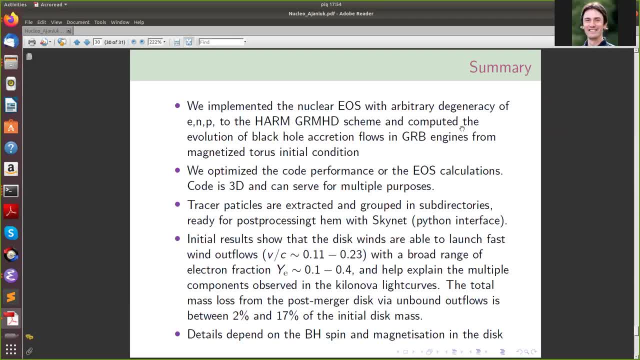 20,000.. Yeah, So it's long, I think. Yeah, yeah, Okay, Thank you, Thank you. Computation time two weeks on this supercomputer? Yeah, yeah, Just to get an idea of Yeah. 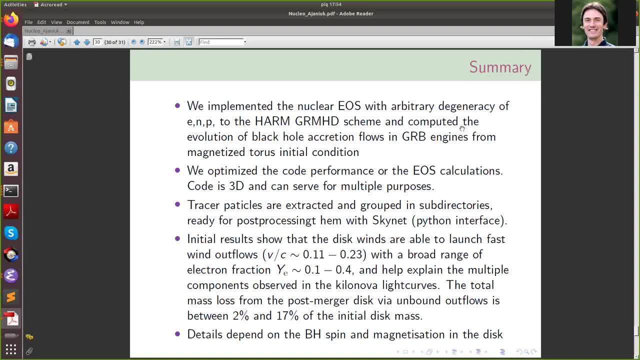